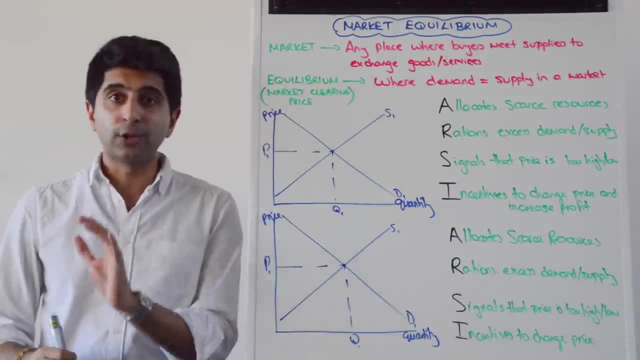 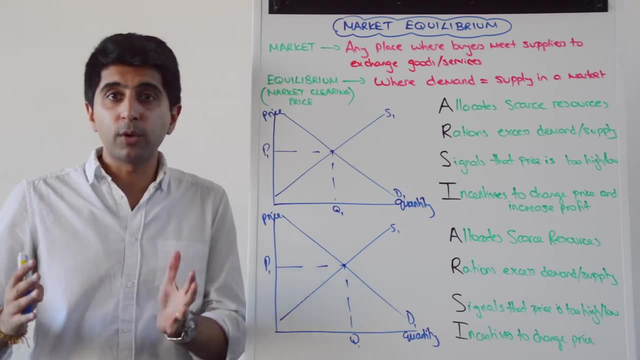 Within markets we get prices and quantities, and those prices and quantities can be derived from the equilibrium in the market. Equilibrium is just the Greek word for balance right, So apply that to a market. it occurs where demand equals supply in a market. 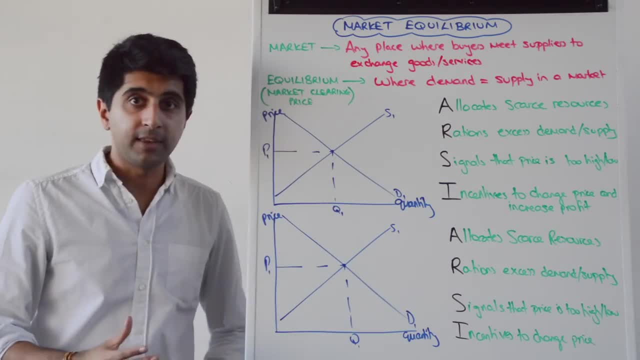 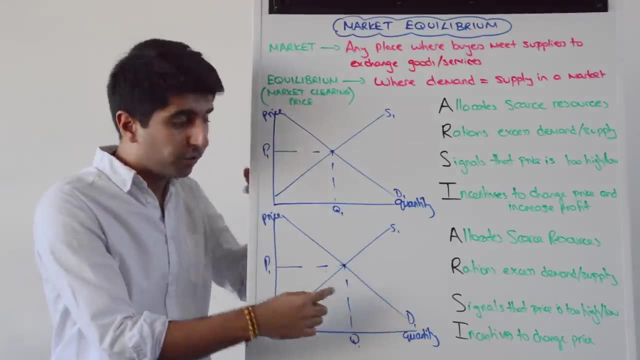 Where demand equals supply. Now, as you can see, I've drawn two diagrams here. I've drawn supply and demand Where the two cross, so where demand equals supply, that's where I've taken the price and the quantity in both cases. 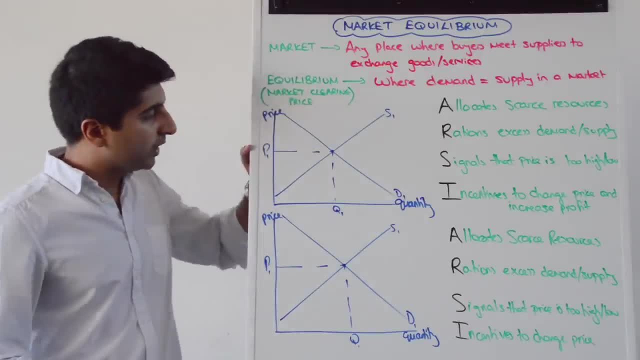 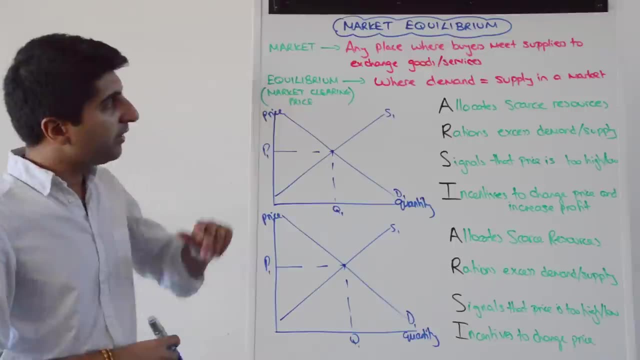 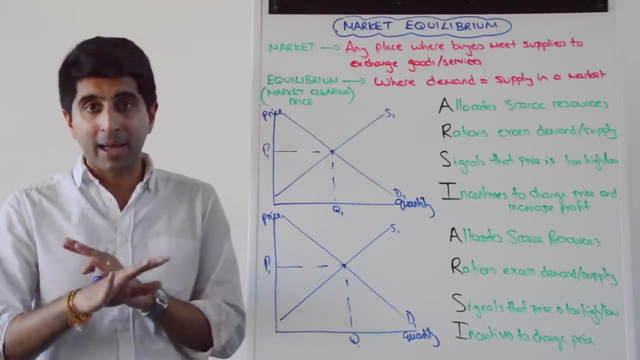 There are other names that we can use here. So we can call P1 the equilibrium market price. clearly We can call Q1 the equilibrium market quantity, Another name for equilibrium. we can say: it's the point where the market clears. So the market is clear from excess demand and excess supplies, ie there is balance between demand and supply. 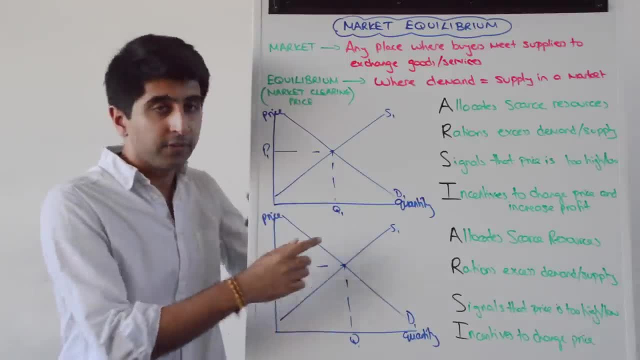 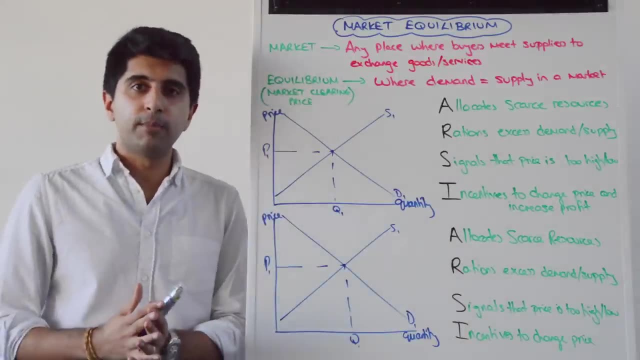 And we can call P1 the market clearing price. We can call Q1 the market clearing quantity- Good to know that jargon as well. So that's what equilibrium looks like. What does disequilibrium mean? Well, clearly, disequilibrium will be where demand does not equal supply. 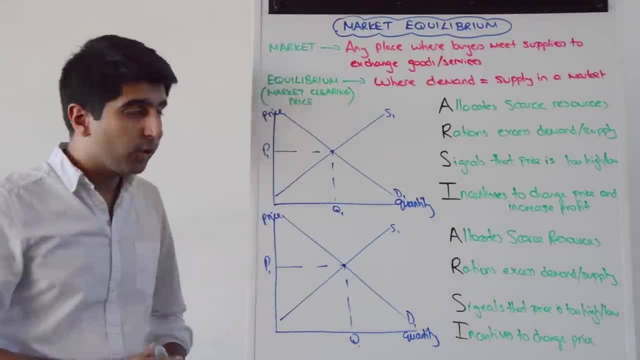 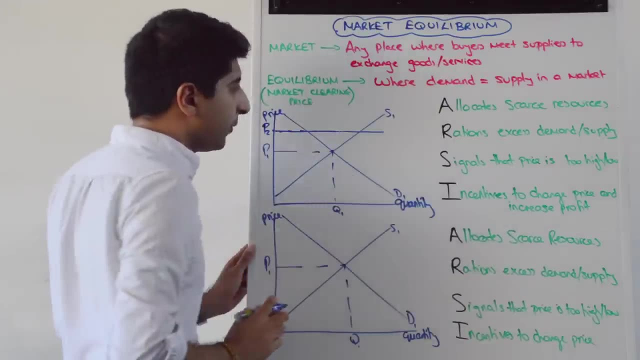 So maybe the price is above P1,, maybe the price is below P1.. If the price is above P1, we'll have something like this, won't we? So the price is at P2, it's pretty clear that that's disequilibrium, because demand and supply are not in balance. 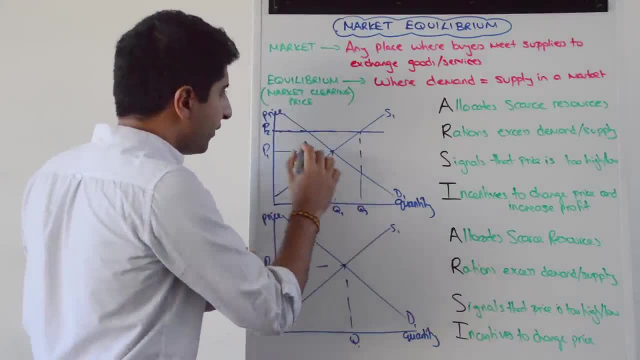 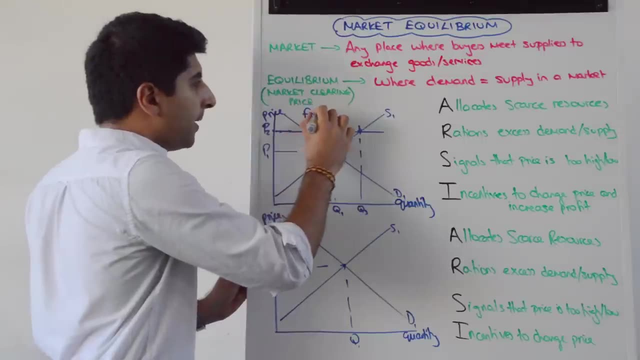 If we take that line across, we can see that supply is over there and demand is over there right. The distance between A and B is excess supply. So supply is clear. It's clearly much more than demand. Well, that's not equilibrium, because equilibrium is relatively equal. 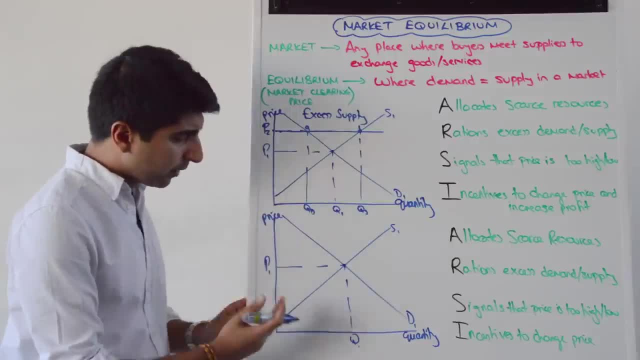 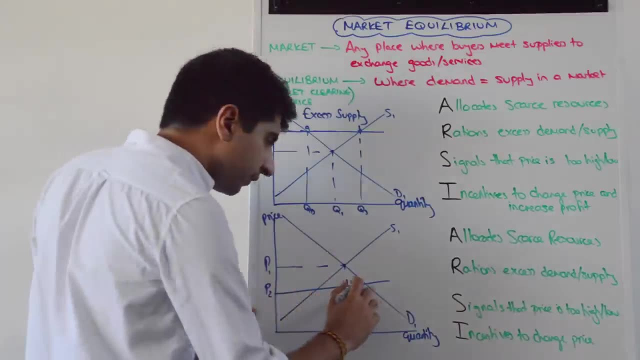 So this is disequilibrium. What about if the price is below P1?? So the price is below P1, let's say here, let's call that P2.. You can see, if we take this line across, that quantity demanded is over there, quantity supplied is only over there. 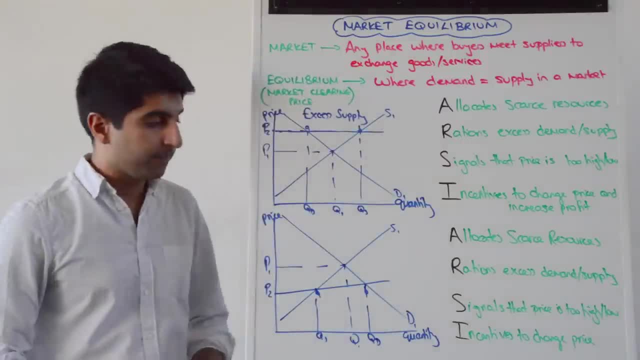 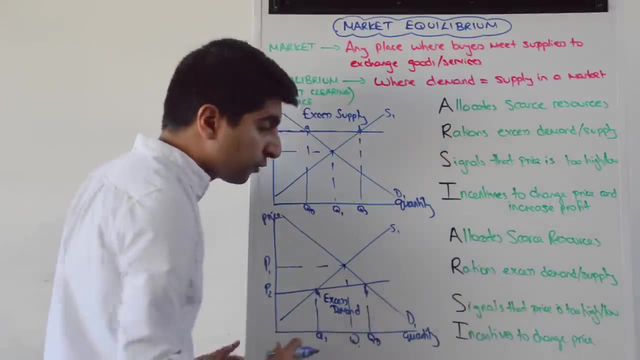 So again we have a problem here. This time demand is much greater than supply. We call that excess demand, Excess demand. This is clearly disequilibrium, because demand is greater than supply. The two are not equal. Demand is greater than supply. 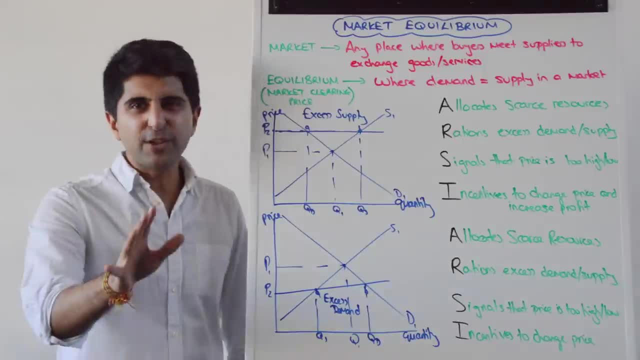 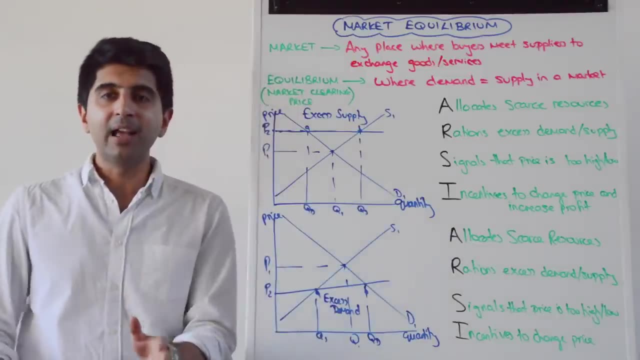 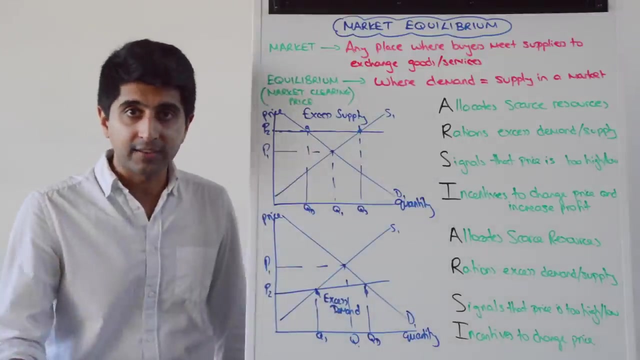 But what's also really, really, really good to know, very useful to know at this stage, is that in a free market, disequilibrium will never last, And that is because the market has got these incredible functions that can take away any problems that exist in the form of excess supplies or excess demands. 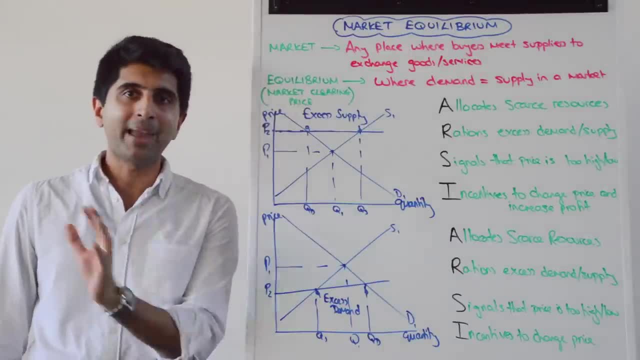 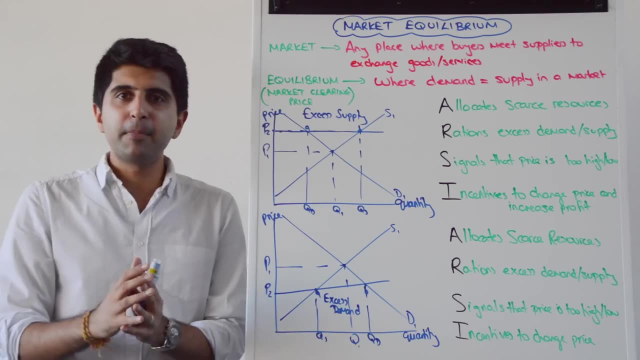 Another name for a market, guys, is the price mechanism, And the price mechanism has got four functions to it, And you can see it here. There is a lovely memory device to remember all these four functions. Just remember RC. The market is RC. 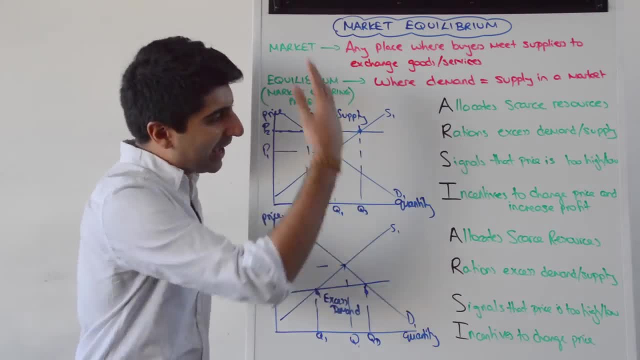 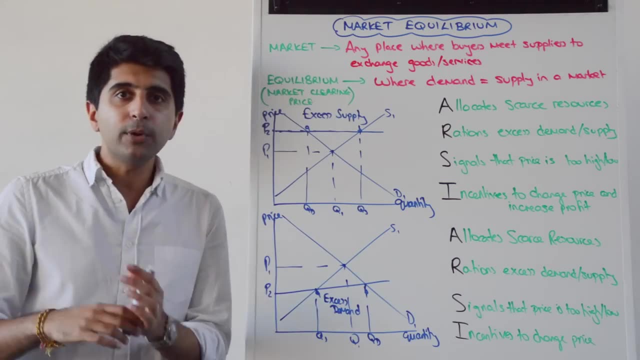 A bit like you guys in the morning, right RC, But yeah, just learn it as RC. Great little memory device And I will give you the four key functions of the price mechanism. The A- the market- will allocate scarce resources efficiently, effectively, at equilibrium. 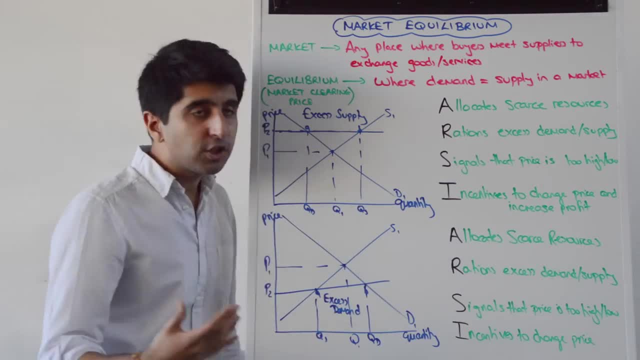 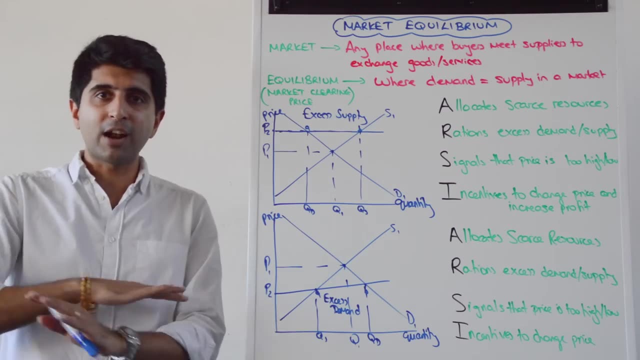 So it allocates scarce resources. How Well it rations away any excess demands and excess supply. So if there are any problems like this excess supply, like that excess demand, it will be taken away, rationed away. How Well signals will be provided. 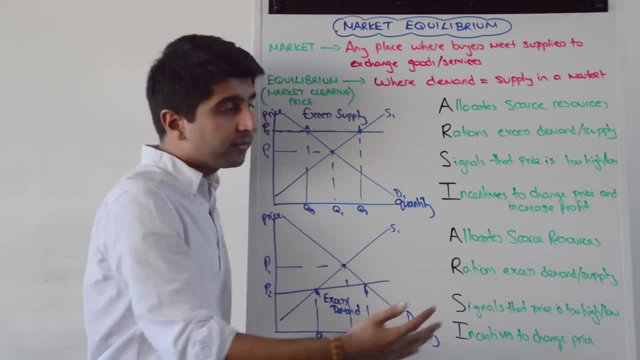 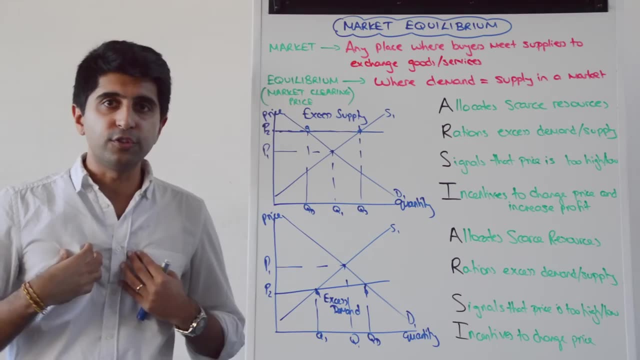 So the price mechanism will send signals to producers That prices are wrong- Prices are either too high or too low- And also the market mechanism. the price mechanism will provide incentives to producers to change prices in order to make more profit. These are the four functions. 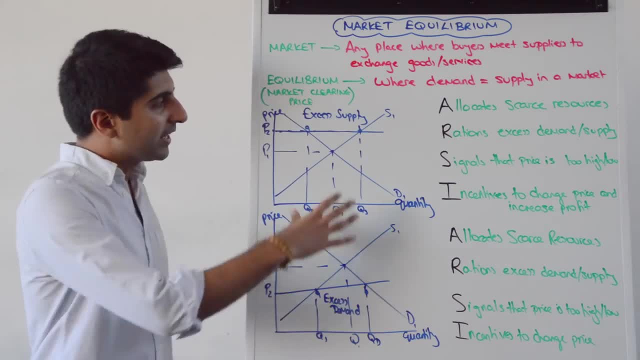 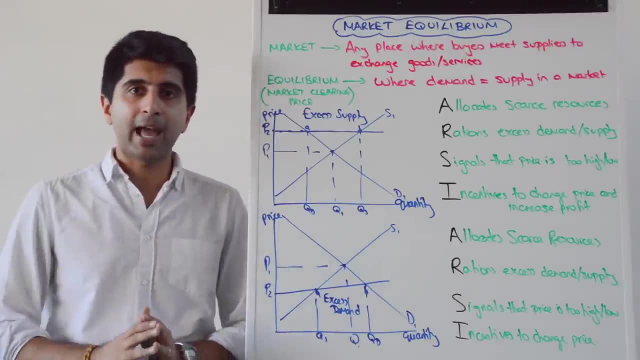 Let's understand how the operation of these functions can take away problems of disequilibrium in a free market. A free market, guys, is when there is absolutely no intervention by government at all. There is no involvement of government, It's just the interaction of producers and consumers. 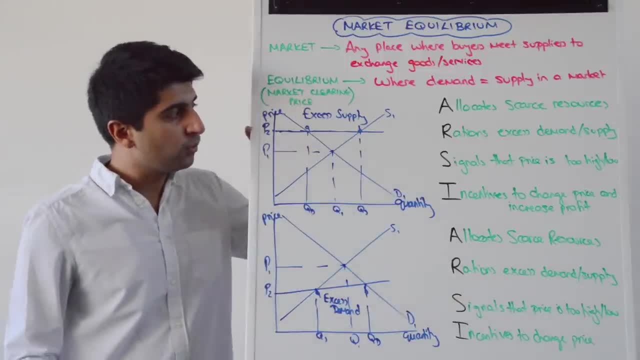 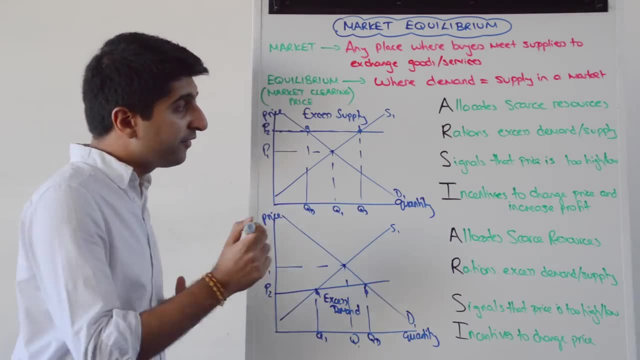 That's it. So in a free market, a price of P2 and the issue of excess supply would not last. Why? How do the functions of the price mechanism get to work? Well, the first thing that happens is that a signal is sent to producers that this price is too high. 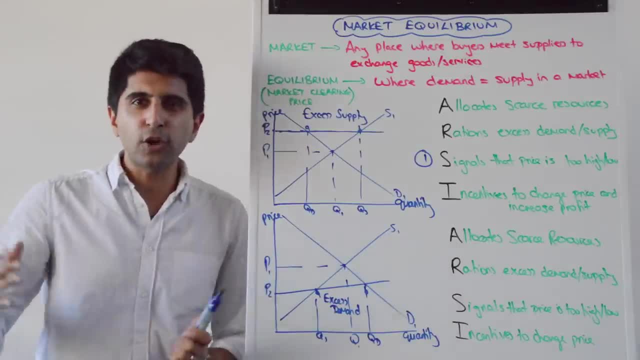 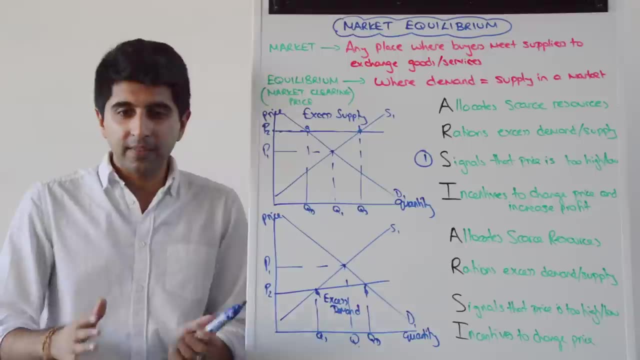 How do producers know What is the signal? Well, they see excess stock in their warehouses. They see their shelves in their shops, you know, are full of stuff It's not being sold. If it's a restaurant, they see that their tables are constantly empty. 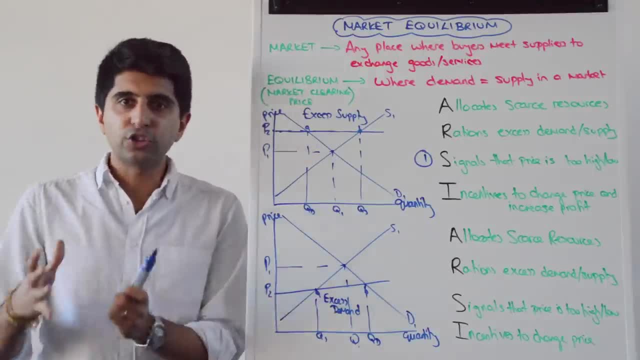 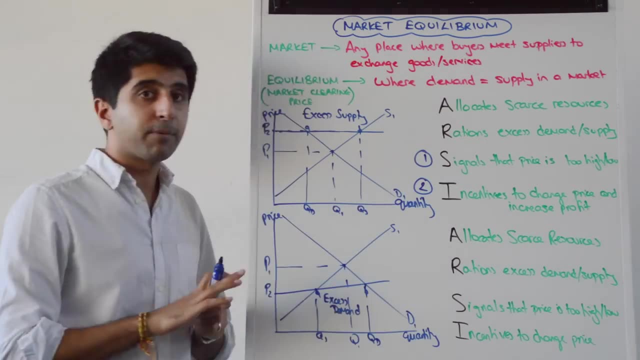 All the ingredients are left in the kitchen, It's clear that they're not shifting their stock. It's a sign that the price is too high. So then the market provides an incentive to producers to change their price, In this case to reduce their price from P2 to P1.. Why, If they reduce their price, they can sell a lot of that excess supply, that excess stock, and make profit from it. Absolutely So that's the profit motive to change price, In this case to reduce price from P2 to P1.. Sell some of the excess stock and make profit. If they do that, what will happen? So if they reduce their price from P2 to P1, there will be a contraction along the supply curve and an extension of demand. So we move along the supply curve downwards: a contraction of supply and a movement down the demand curve- an extension of demand. 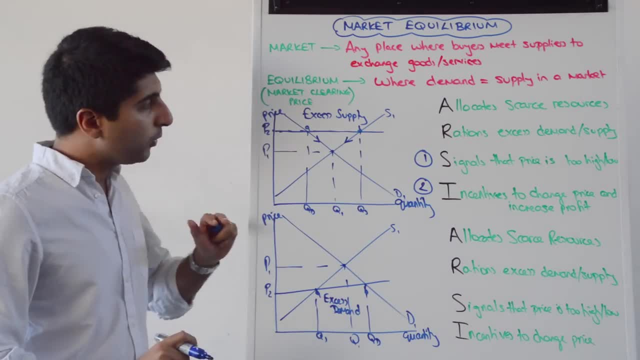 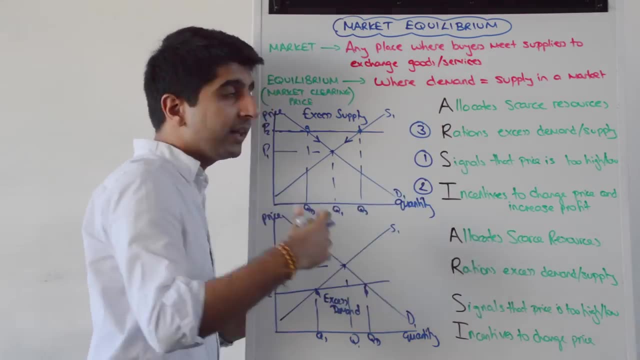 And we get to P1 and a quantity of Q1.. At P1 and Q1, we're back in equilibrium right, And here there is no excess supply and no excess demand. We've rationed away the excess supply. That was the issue. 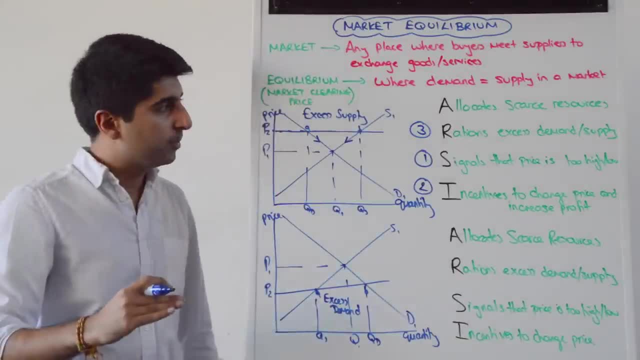 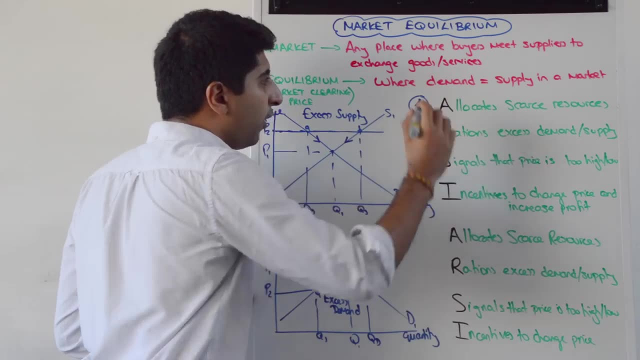 Completely rationed by these movements. as the price has been reduced And at P1 and Q1, because there are no excess supplies and no excess demand, we have a perfect allocation of scarce resources. We're going to look at that in way more detail. 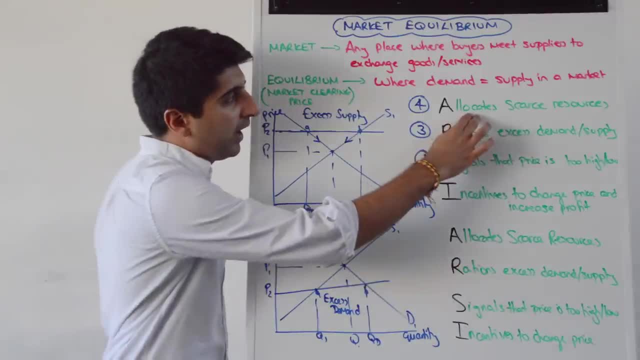 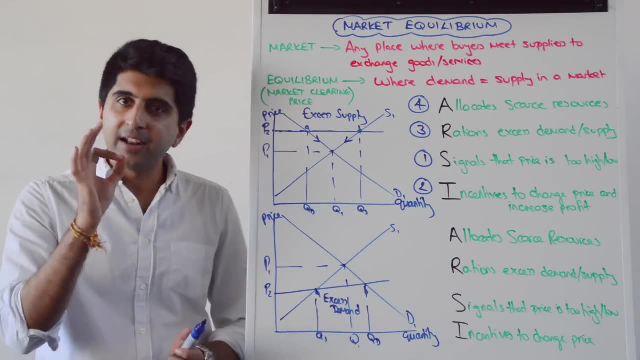 If you go to a later video in the playlist, you'll see how I analyse what I mean by a perfect allocation of scarce resources in more detail. But basically, where we're in equilibrium, that is a perfect allocation of scarce resources, Great. 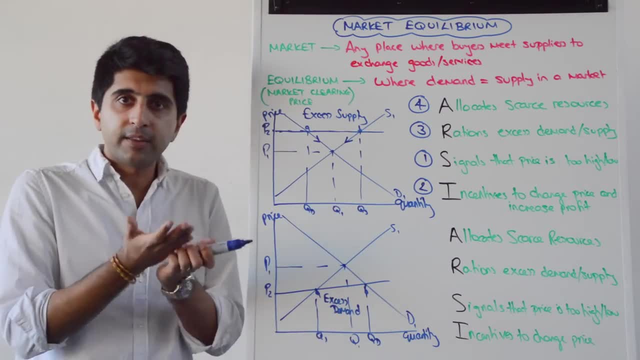 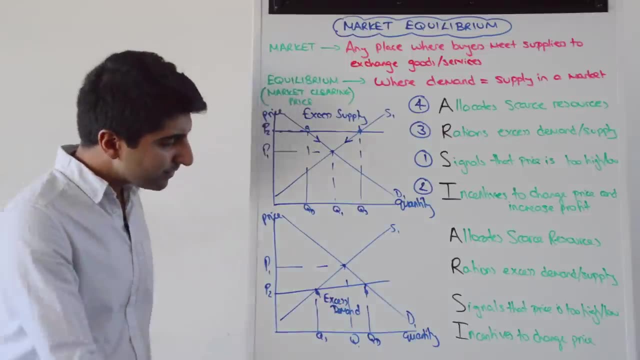 So in a free market, any time there is excess supply, if the price is above equilibrium, that will be taken away through the functions of the price mechanism, Through RC. What about if the price is below equilibrium? here We can see there is an excess demand. Well, exactly the same order. First, a signal will be sent to producers that now the price is too low. How will producers see this? Well, there will be massive queuing for the good or service. There will be huge waiting lists for consumers to buy the good or service. Maybe there will be huge competition between buyers to get this good or service. A clear sign that the price is too low There is this excess demand. Supplies can't keep up, basically. So then there is an incentive for producers now to increase their price from P2 to P1. 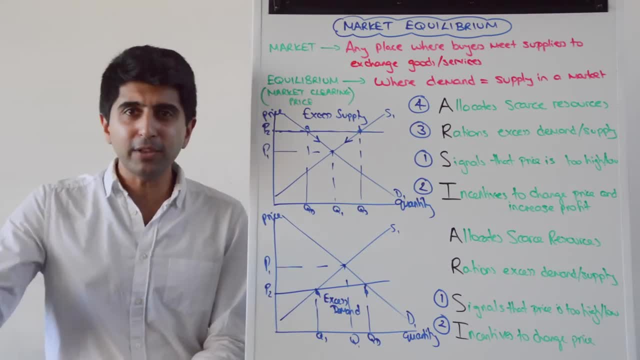 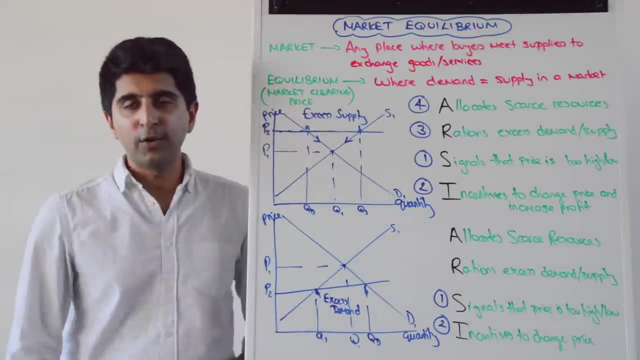 Milk it. If you've got a huge demand for your product, milk it, Raise your price, Satisfy some of that extra demand by producing more at a much higher price- A great way to increase your profits. Obviously, you wouldn't say milk it, but that's a basic idea, isn't it? Milk it. You've got a huge demand. Push up your price, Make a higher profit from that extra demand. So there is an incentive to increase price here in order to increase profit for the producer. If that happens, so from P2 to P1, the price is raised. 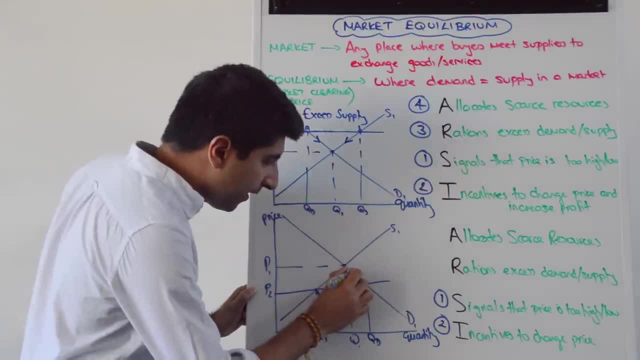 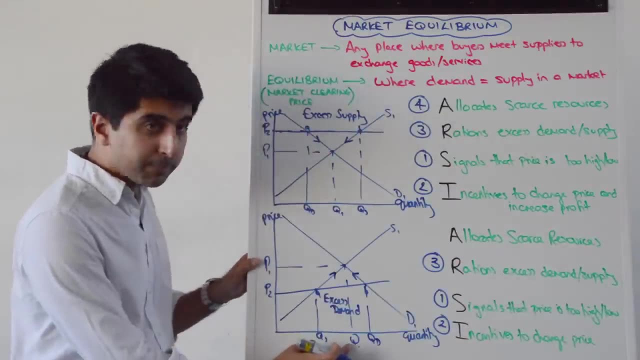 You can see that there is now an extension of supply and a contraction of demand And we end up at P1, which means that the excess demand has been rationed away. We end up at P1 and Q1.. Perfect equilibrium, No excess demand.